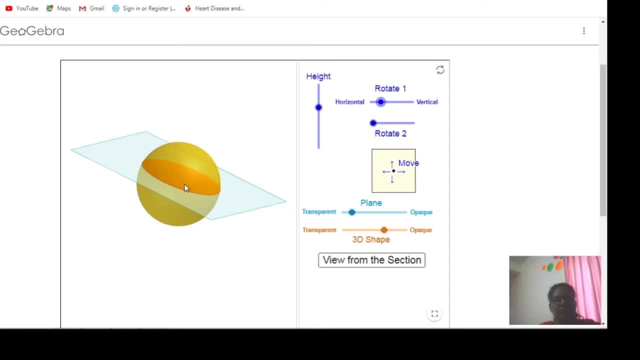 And this is the plane And this is the plane. dark portion, or the boundary of this. dark portion is the set of common points on the sphere and plane and which is nothing but a circle. so these are the different circles. if you change the position of plane, that is, we will get the different planes. 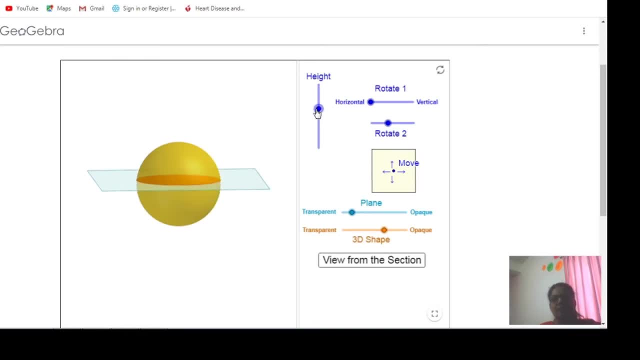 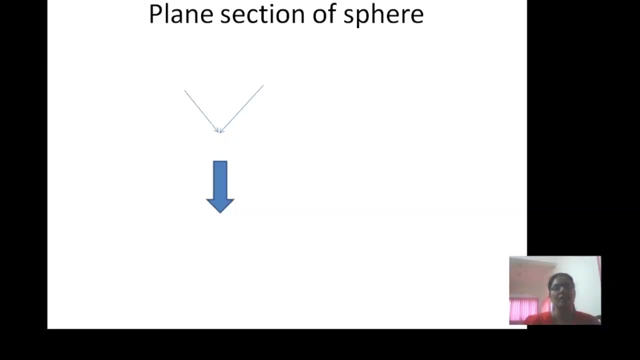 and the intersection of plane and sphere is nothing but a circle. so view from this section. so if you consider here the plane and the sphere and set of common point is nothing but a circle. so, as we have seen in the video, intersection of sphere and plane is a circle. 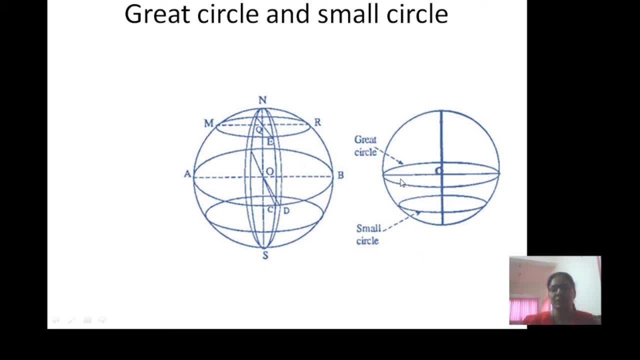 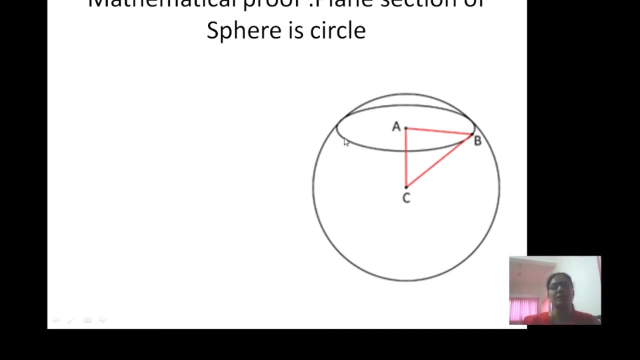 if the plane is passing through the center of the sphere, then the plane section is a circle and that circle is called the great circle. otherwise the circle is called the small circle. so now we will see the mathematical proof, for the plane section of a sphere is a circle. 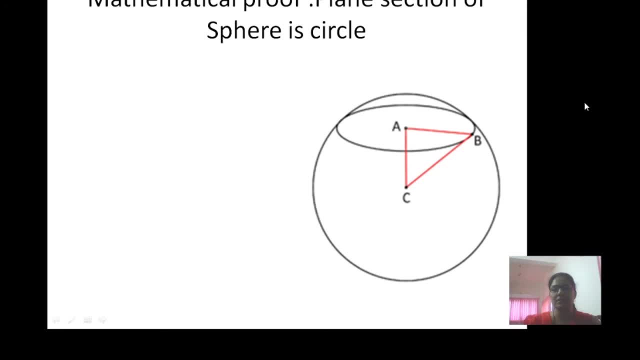 for that we consider a sphere with center c and say radius r, so let capital b, an arbitrary point on the plane section of the sphere. so we draw a perpendicular from point c on the plane, say c a. so a is the plane of, a is the foot of perpendicular, as the segment c a. 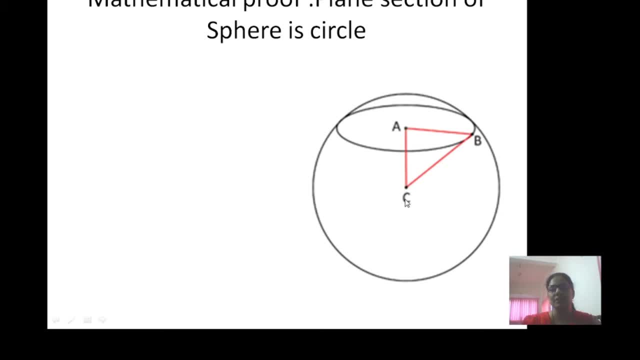 segment c a lies on the plane, so the segment c is perpendicular to a- b. so now here, c is a fixed point because it is the center of the sphere. a is also here fixed point. so distance: c a is a fixed distance and c? b is also fixed distance because it is a radius of the sphere. so now, since this triangle, 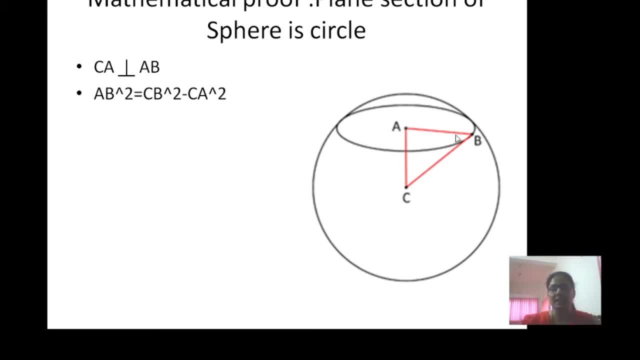 is a right angle triangle. in this right angle triangle we use the pythagoras rule, so we get here: a b square equals to c b square minus c a square and, as we have discussed, these two points are fixed points. so the distance a- b: by using this distance a b, we get a b square and b b square. 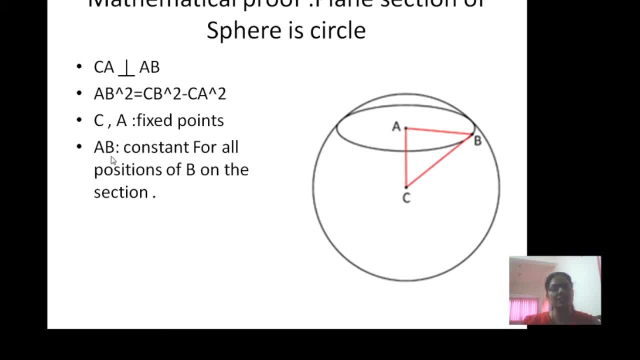 this relation we can say that it is a constant distance for all positions of the point b on the plane section. here a is a fixed point distance, a, b is fixed for any a, any b on this plane section. so by definition of circle the locus of b, that is, the plane section of the sphere, is nothing but a. 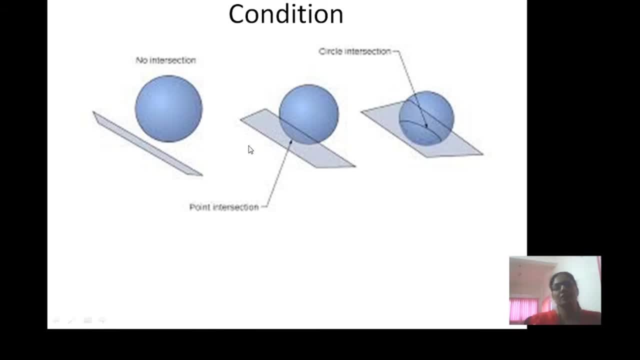 circle now. next we will see what is the condition so that the given plane intersect the given sphere. so, as we know that there are three cases: either the plane inter plane do not intersect the sphere. second, plane intersect the sphere at a single point and second in circle. third, one is in circle. 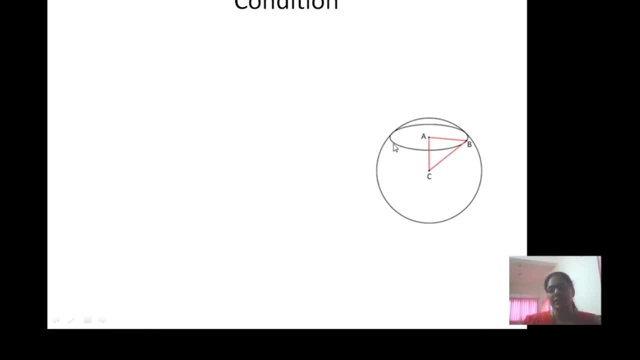 so now it's here. find the condition. we consider a sphere with center c and c, radius r. so see, in this case the plane intersect the sphere and here we can easily see, see that the distance c is less than r. so if the given plane intersect the sphere, if, and only if, the distance c is less than equal r, that is the radius of the sphere. 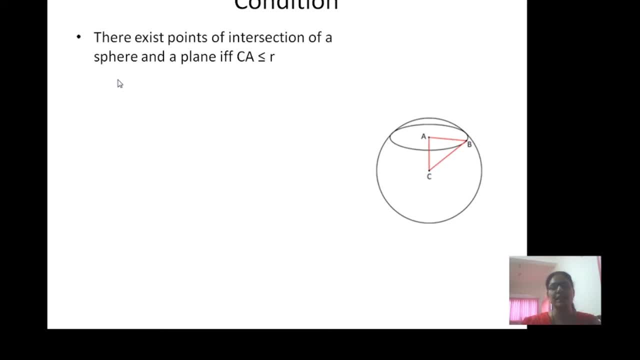 there exists points of intersection of r sphere and the plane if, and only if, distance c is less than equal r, that is, if, and only if, c a square is less than equal r square. now next thing is we have to find this distance c a. so for that we consider the equation of: 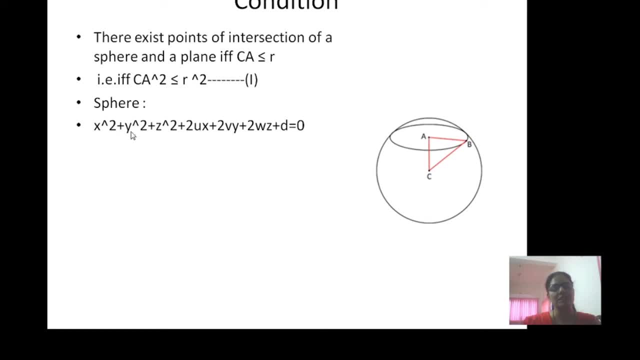 sphere in general form. suppose the equation is x square plus phi square plus z square plus twice ux plus twice v, y plus twice w, z plus d equals to zero. then the center of the sphere is c minus u minus v minus w and radius is square root of u square plus v. 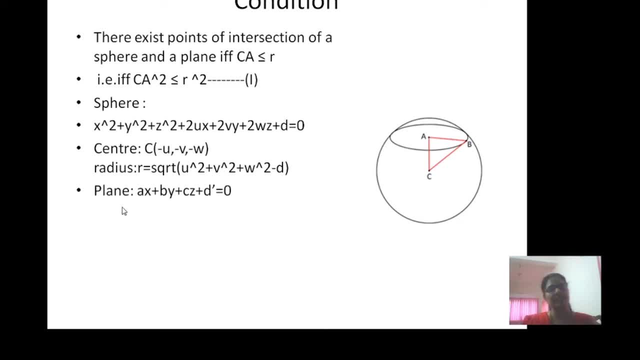 square plus w, square minus v. the next, consider the equation of plane, and x plus by price, is that plus d equals to 0. so now, here we know that the distance c is nothing but the. this distance c, a is the distance of the center of the sphere from the plane, and there is one formula to find the. 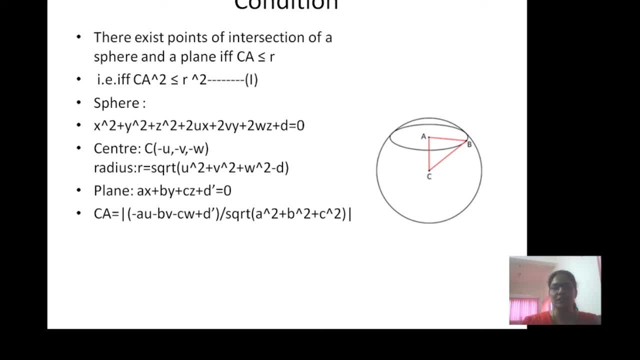 perpendicular distance of the point from the plane. so use the same formula. So here distance c is equals to mod of minus au, minus bv, minus cw plus d, dash divided by square root of a square plus b square plus c square. So this gives the distance of the 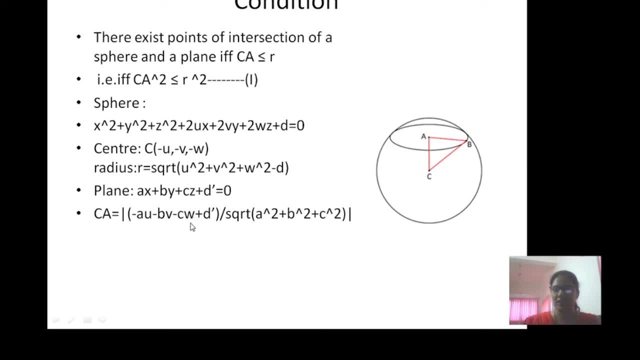 center c from the plane. Just squaring this, we get here c square. Now put the distance c square in equation 1 and solving we will get the required condition. This distance can be written in this form: Just put it and solving we will get the condition. 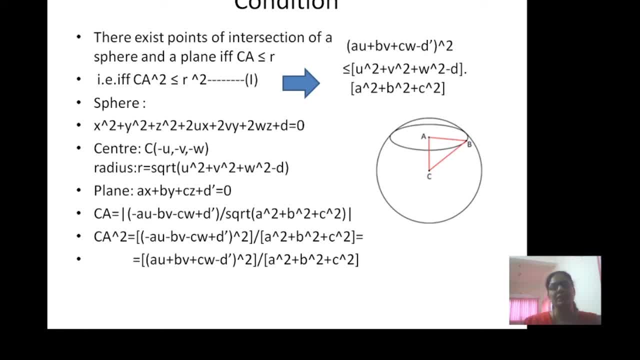 for that the given sphere and plane intersect to each other, and that condition is au plus bv plus cw minus d. dash bracket square is less than equal u square plus v square plus w square minus d, into a square plus b square plus c square. So suppose we have to, given the equation of: 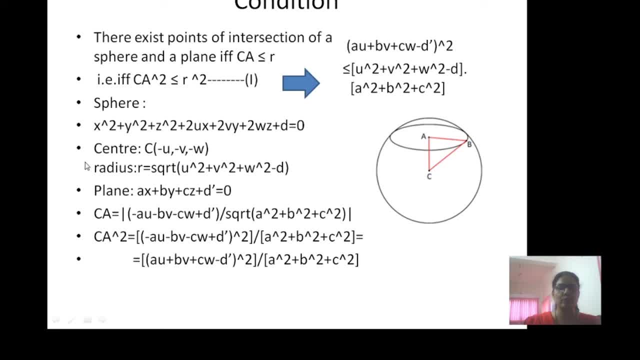 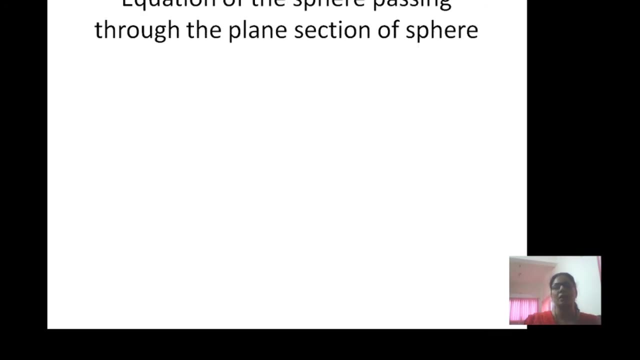 sphere in general form, as well as the equation of plane. Using this condition, we will check whether there is a point of intersection between the sphere and the given plane. Okay, as we know that the plane section of sphere is a circle, So now, next, we will see what is the equation of sphere which is passing through this circle. 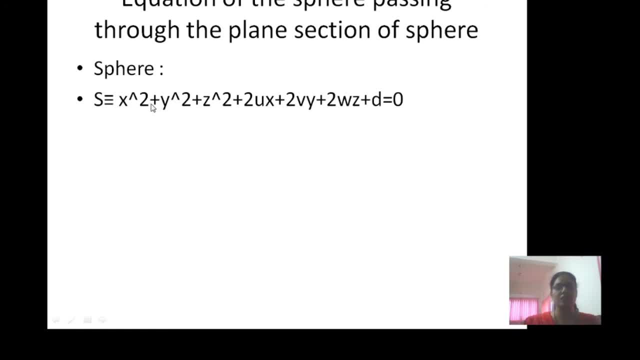 So for that consider the equation of sphere in general form, Equation of plane as ax plus by plus cz plus d, equal to 0. Then we know that the intersection of the plane and sphere is circle if they are intersecting to each other. So equation of sphere passing through the 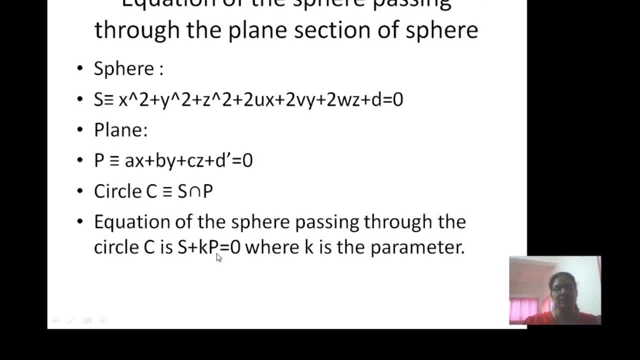 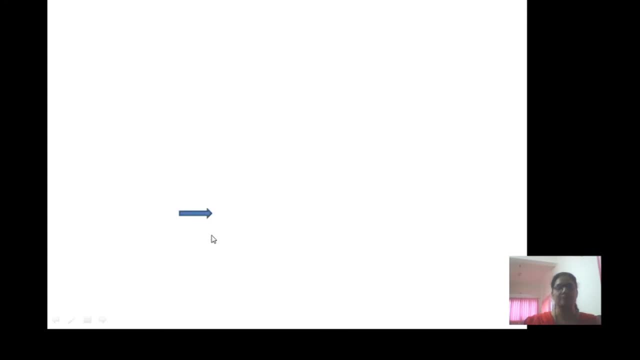 circle c Is x plus kp is equals to 0, where k is a parameter. You can easily prove that this equation is the equation of sphere which passes through the plane as well as the given sphere. Similar example on this example is: find the equation of sphere which is passing through. 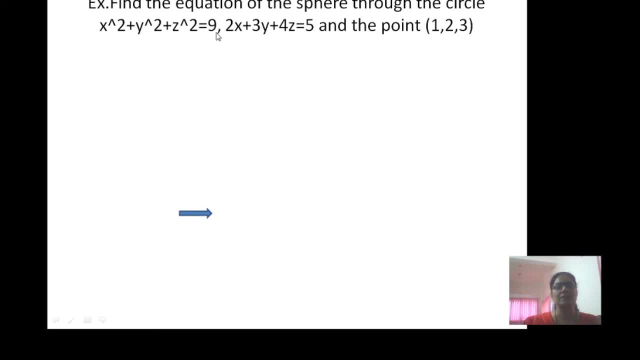 the circle x square plus pi square plus z square equals to 9, and 2 x plus 3 y plus pi 4z equals to 5.. We know that a sphere together with plane represent a circle and point 1 to 3.. 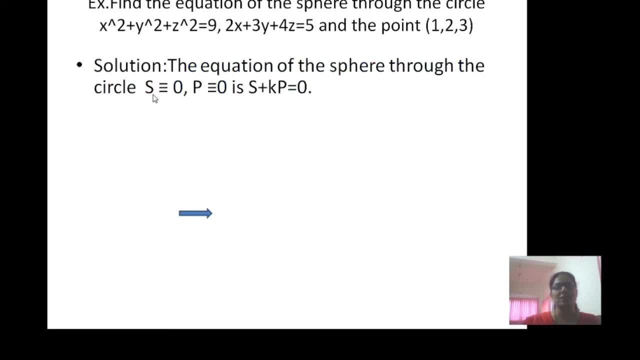 So, as we know that the equation of sphere which, passing through the circle x, s equals to 0 and p equals to 0, is x plus k, p equals to 0. Here, k is a parameter and we calculate this parameter by using the another geometrical condition. So the equation of 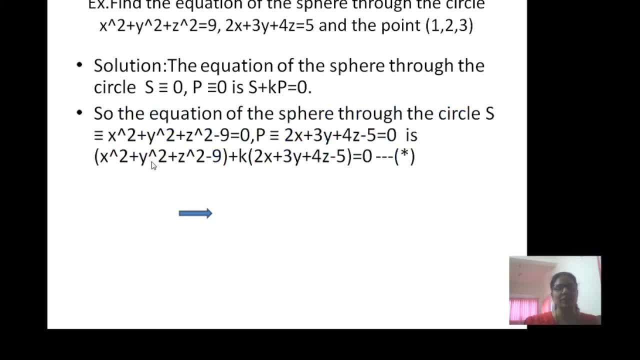 required sphere is x square plus y square plus z square minus 9 plus k times 2x plus 3y plus 4z minus 5 equals to 0.. Because we have given the sphere denoted this part as s Next p is 2x plus. 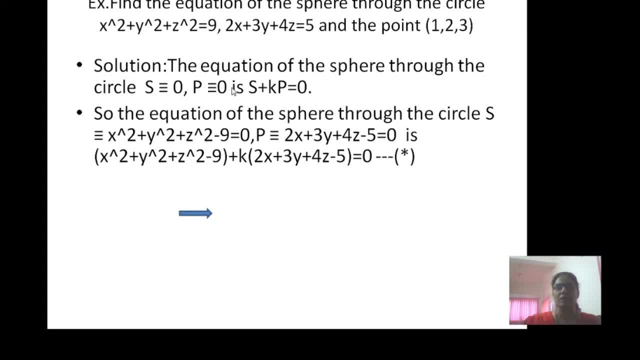 3y plus 4z minus 5.. Put in this equation So we get the required equation of sphere. One more condition is given that the required sphere is passing through the point 1,, 2, 3. So this point lies on the required sphere. So 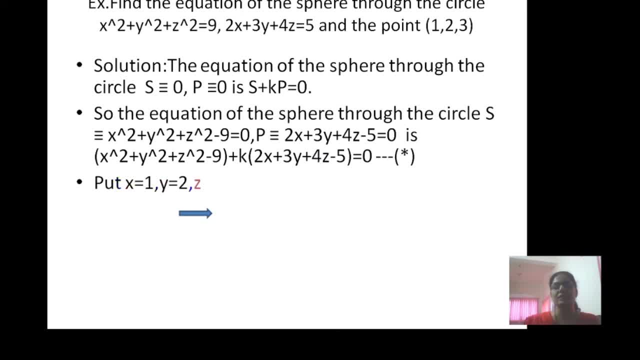 we put here or substitute here, the value of x equals to 1, y equals to 2 and z equals to 3 in equation star, And solving this we get 5 plus 15k is 0.. Solve this equation for k. So. 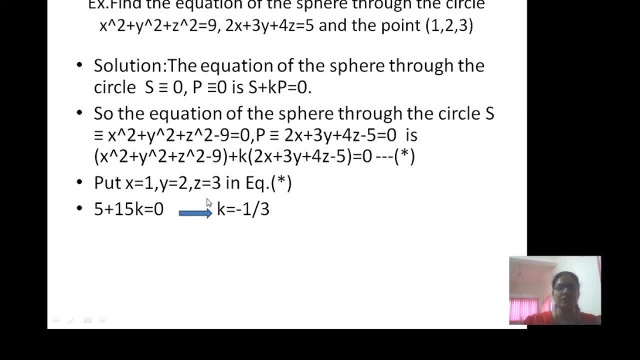 we get here k equals to minus 1 by 3.. Now put this value of k equals to minus 1 by 3 in equation, So we will get the equation of required plane, And which is 3x square plus 3, into y square plus. 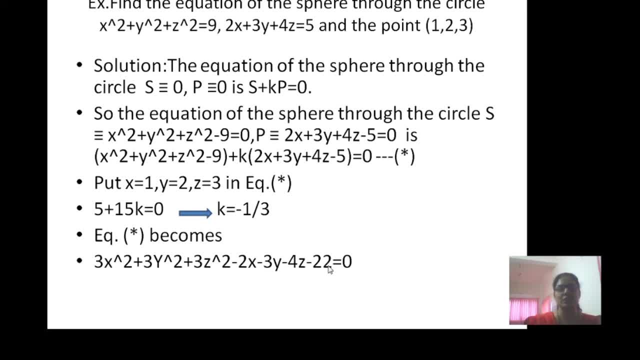 3 into z square minus 2x minus 3, by minus 4z minus 22 equals to 0.. Thank you.